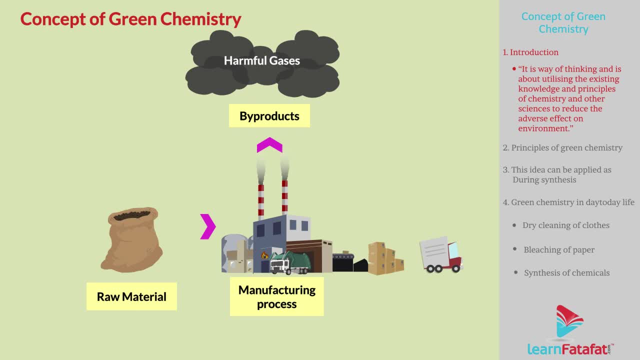 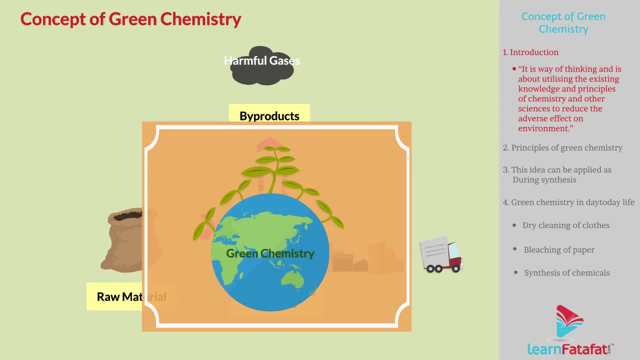 cause pollution in environment. Such process cannot be environment friendly. Also, waste generation and its disposal is not cost effective. So utilization of existing knowledge to reduce the chemical hazard is called Green Chemistry. Environmental hazards promoting developmental activities using by-product and different. 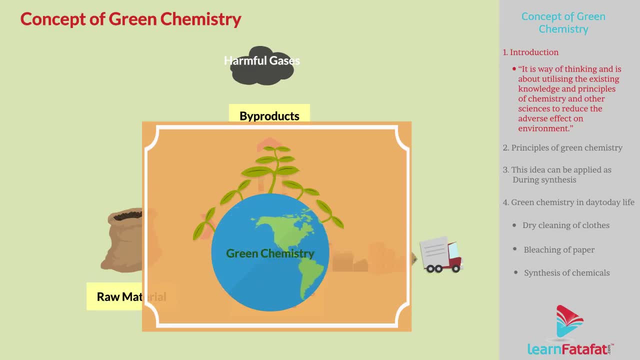 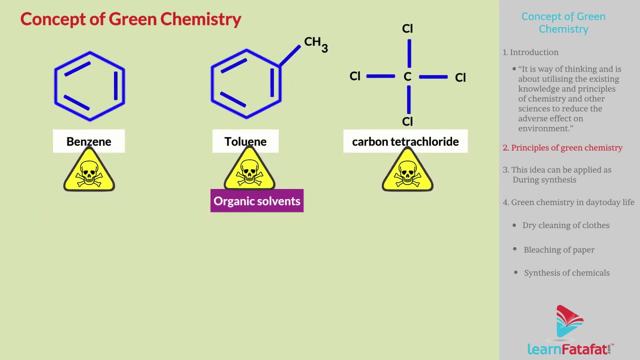 ways is a basis for Green Chemistry. After knowing idea of Green Chemistry, questions arises that how to apply the principles of Green Chemistry. Let us learn it. Organic solvents such as benzene, toluene, carbon tetrachloride, etc. are highly toxic. 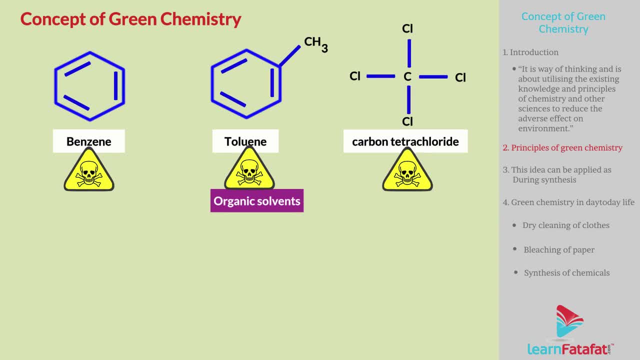 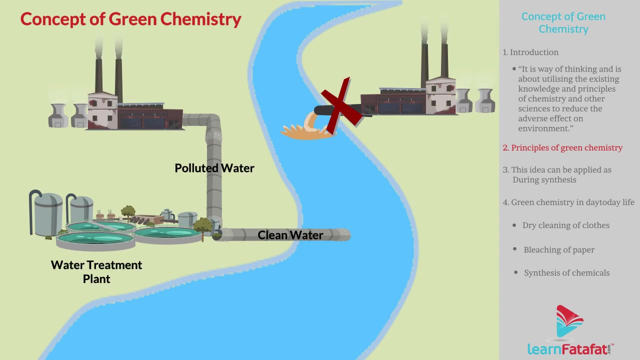 So it is necessary to take precautions during their use. Chemical reactions involves reactants attacking reagents and medium where reaction takes place In chemical reaction. if reactant are fully converted into eco-friendly products in an eco-friendly medium, then there would be no chemical pollutants in environment. 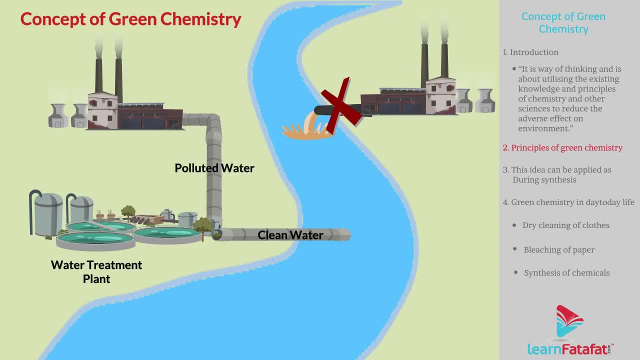 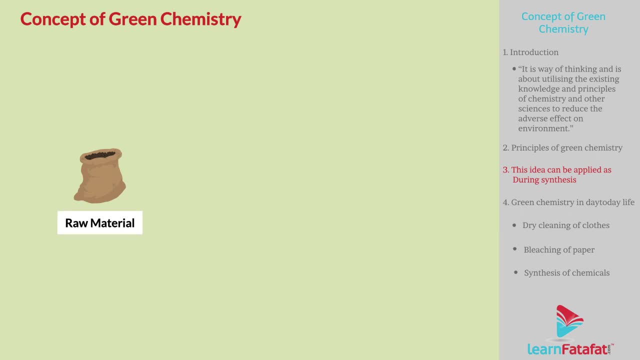 This idea can be applied as during synthesis, reactants or starting material should be chosen in such a way that product yield should be 100%. This can be achieved at optimum conditions of synthesis. Water proves to be good medium for such reaction due to its high specific. 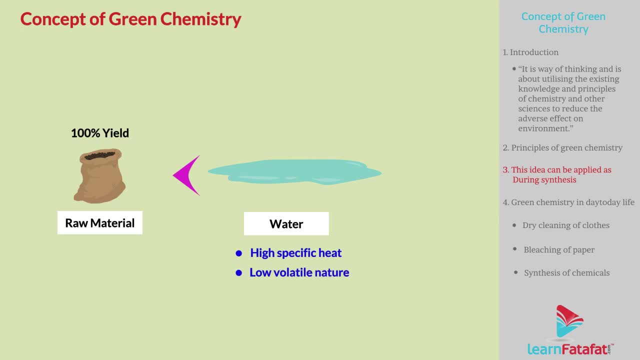 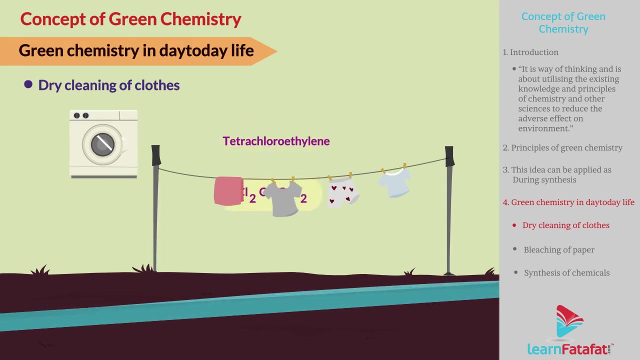 heat and low volatile nature. Water is cost-effective, non-inflammable and is non-carcinogenic. Cream Chemistry in Day-to-Day Life Dry Cleaning of Clothes. Tetrachloroethylene was earlier used as solvent for dry cleaning. This compound, if reaches to groundwater, contaminates it. 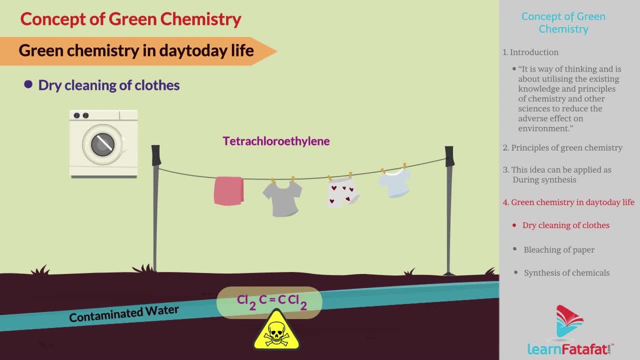 It is also suspected as carcinogen. Now, the process of dry cleaning is now replaced by liquefied carbon dioxide with suitable detergent. Comparably, this results into less harm for groundwater. Nowadays, hydrogen peroxide is used as bleaching agents for clothes in laundry.